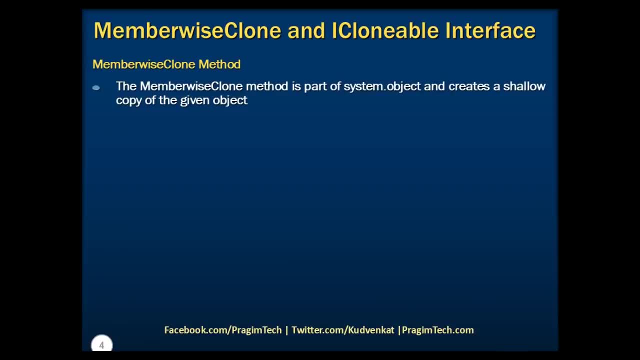 part of systemobject and creates a shallow copy of the given object. Member-wise clone method copies the non-static fields of the chosen object to the new object In the process of copying. if the member-wise clone finds if the field is a value, type a bit by bit copy of the 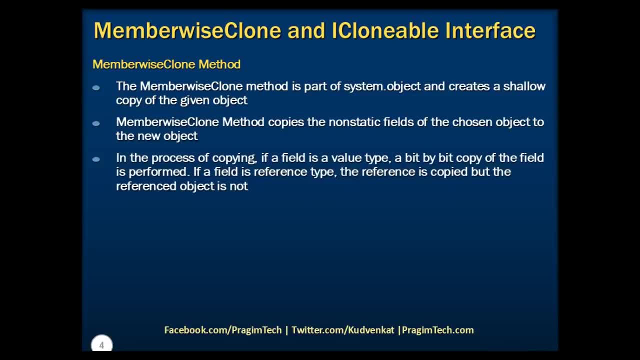 field is performed and if a field is reference type, the reference is copied, but the reference object is not. If you have viewed the previous session, you can recollect that we have demonstrated the value type copying as well as the reference type copying. We strongly recommend you to. 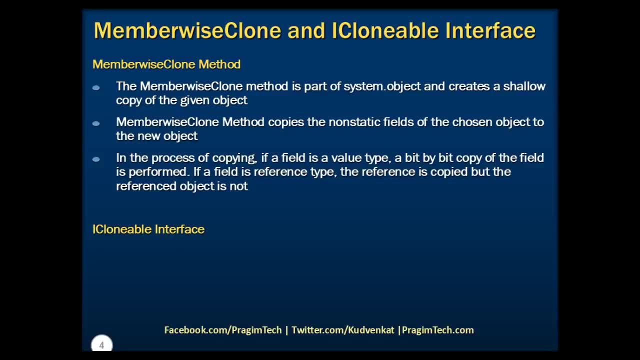 view the previous session of the tutorial before proceeding Now. let's now understand the iClonable interface. The iClonable interface provides with a customized implementation that creates copy of an existing object. iClonable interface contains one member- is the clone method, and that clone method is intended to provide support. 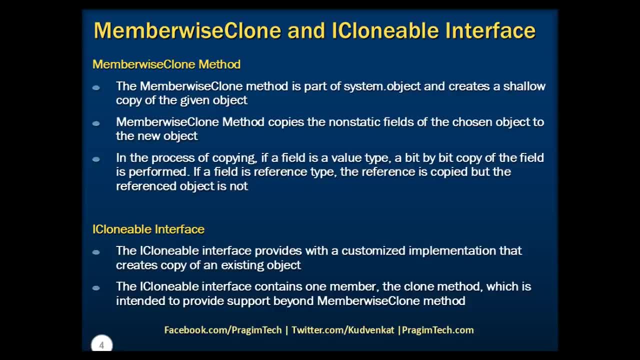 beyond member wise clone method. in some cases, we use clone method and use the member wise clone within the clone method. now, if this is confusing at this moment, don't worry, we are going to discuss this in greater detail using simple example. let's now switch to Visual Studio and see how we can. 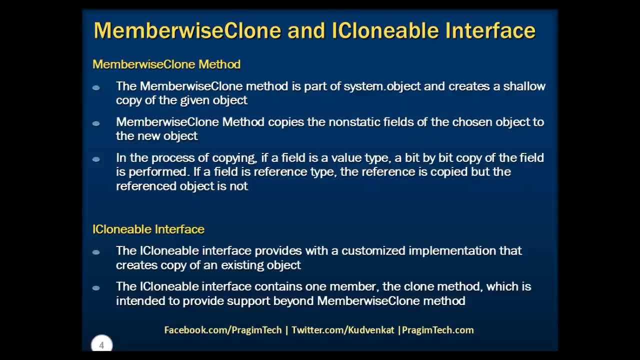 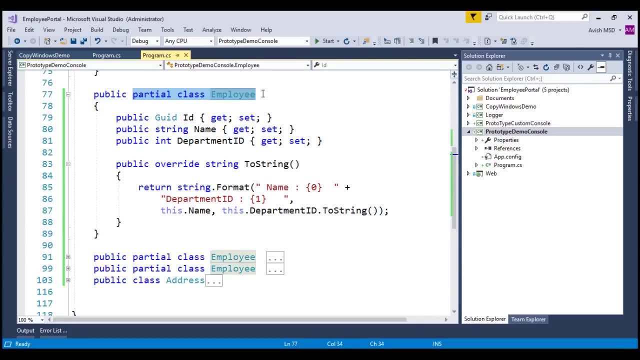 implement the prototype design pattern, using these concepts. to make the things faster, I have already created a console application with a partial employee class consisting of ID name and department ID. I have also created an override to string method to print the employee details. to copy these employee details we need to inherit either. we need to inherit the iClonable. 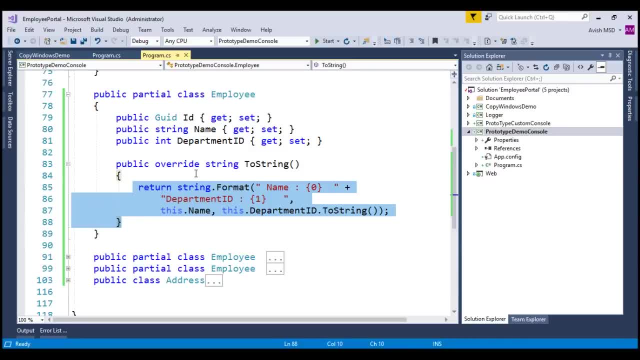 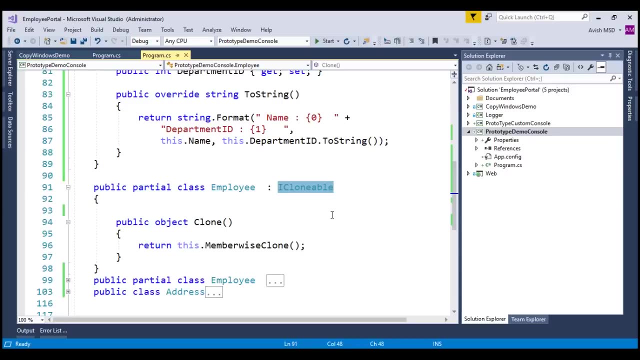 interface or we need to create a custom clonable method. to simplify, I have already created another partial class of the same employee and I have inherited the iClonable interface. if you recollect, iClonable interface will have one clone method which returns the. 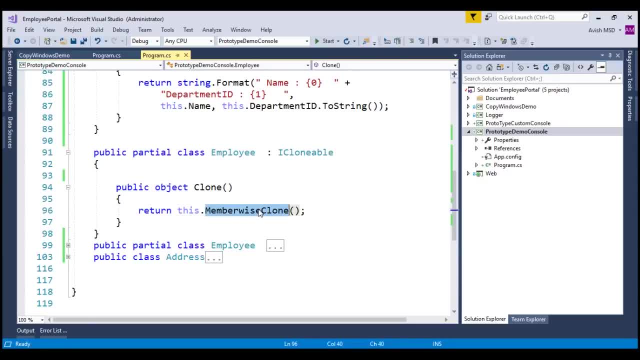 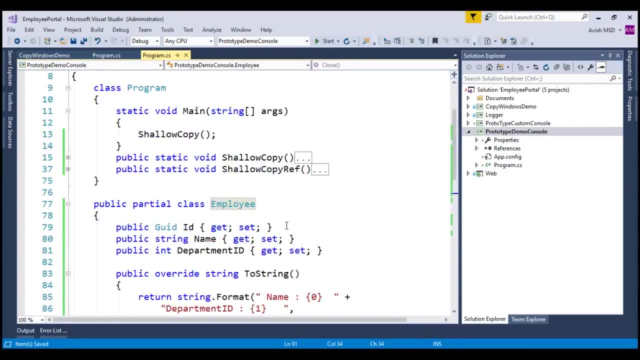 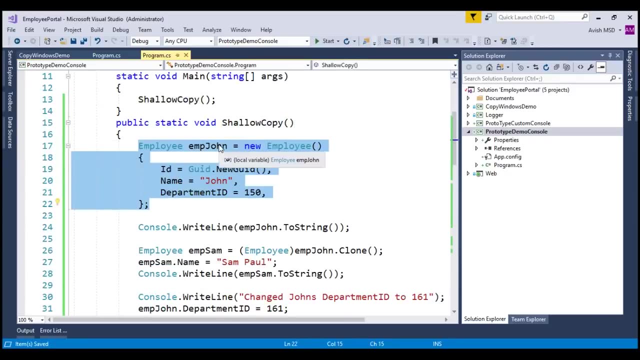 object and I have used the member wise clone to return the current object that is being cloned. in order to test these changes, have created a simple method, shallow copy and created an employee object and named it as John. I have assigned the department ID as 150 to this employee Once the object is created. 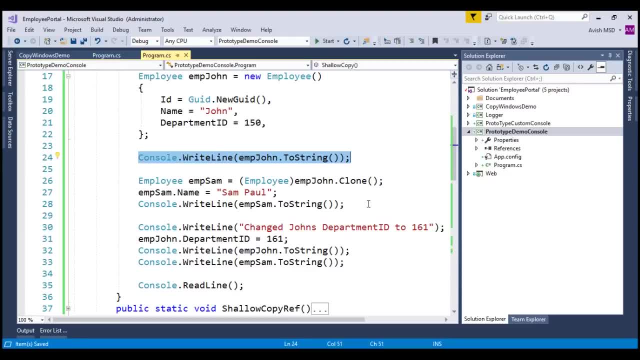 I am printing the details of this employee to the console. In step 2, using the clone method, I have copied the employee John's details to employee Sam and I have changed the name of this employee Sam to Sam Paul, since the copied object consists the name of John. Once that is complete, I am printing the 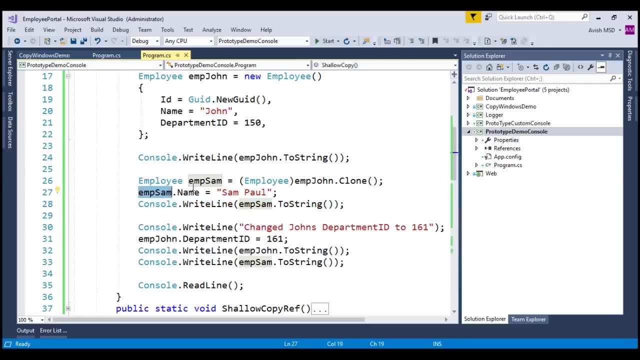 output to a console with employee Sam's details. In step 3 I am changing the employee John's department ID to 161 to see whether this department ID propagates to employee Sam's department ID or the employee Sam's department ID remains the same. 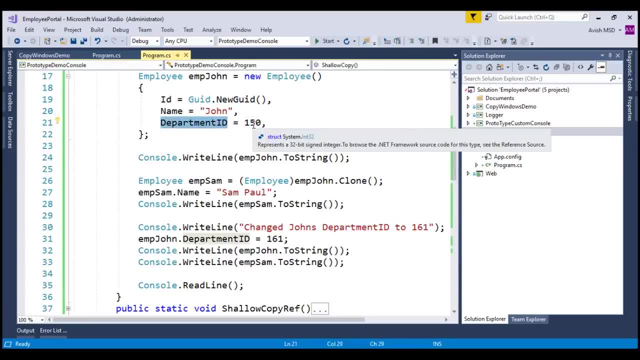 I have changed the department ID as 150.. Ideally it should remain department ID as 150 and the change of these details shouldn't impact employee Sam's details. Let's now run this application. Notice that in step 1, both John and Sam has got the same. 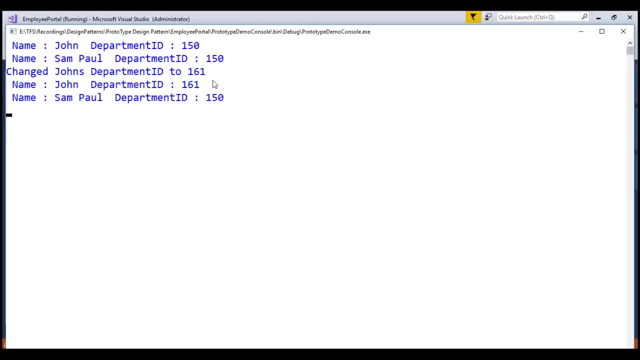 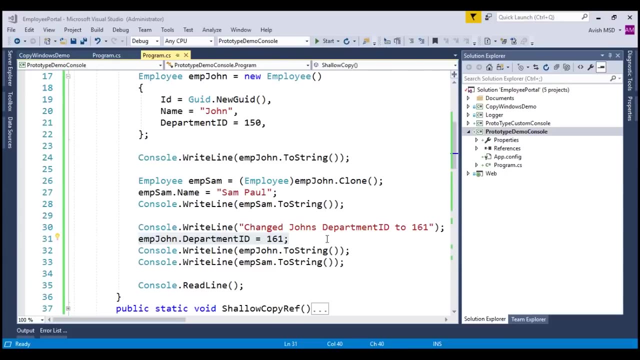 department ID In step 2. once it is cloned and the department ID of John is changed, the Sam's department ID is not being affected. With this we have successfully implemented the simplest shallow copy application. Now let's switch back to the application. Now let's say we need to enhance this employee object to hold the address details. 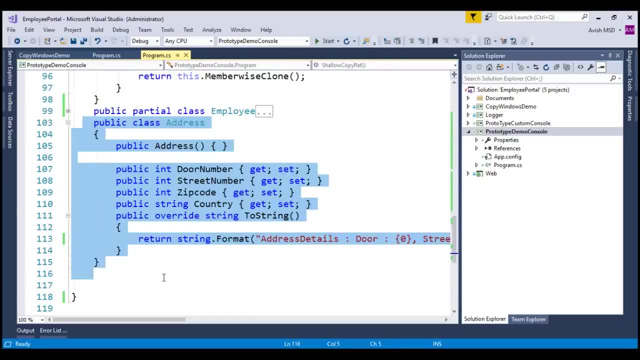 In order to do that, I have created an address object with door number, street number, zip code and country. I have also overridden the to string to print the address details of the employee. Now I have extended the partial class employee and added the address. 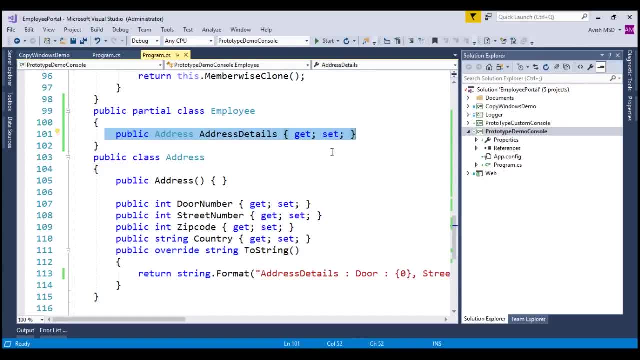 details. in the beginning of this session we have discussed that member wise clone copies the object reference if the field is of reference type and it does not copy the reference object itself. in our case, address is a field of employee object and is a reference type in order to 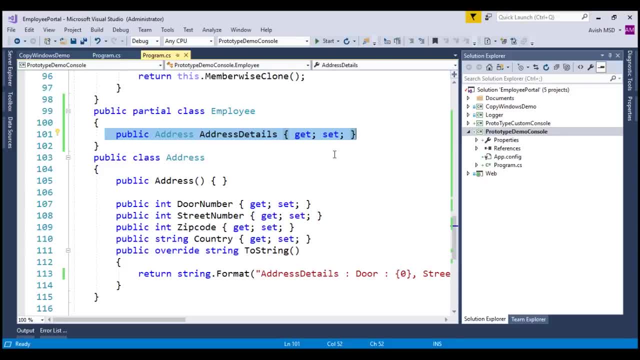 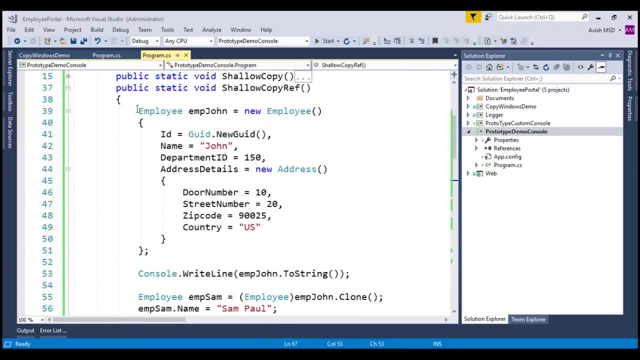 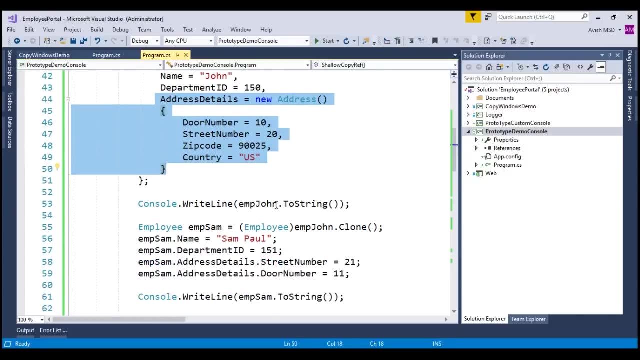 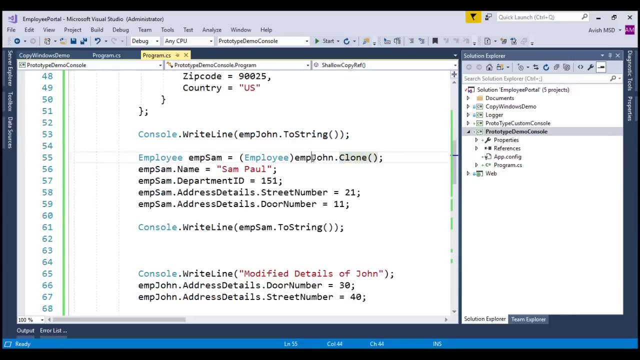 verify if the address is referenced for the copied employees, i have created another method called shallow copy reference. in step one of this method, we have created an employee named john, along with the additional address details. once employee is created, we are printing the employee details to the console. in step two, we are cloning the employee john and copying. 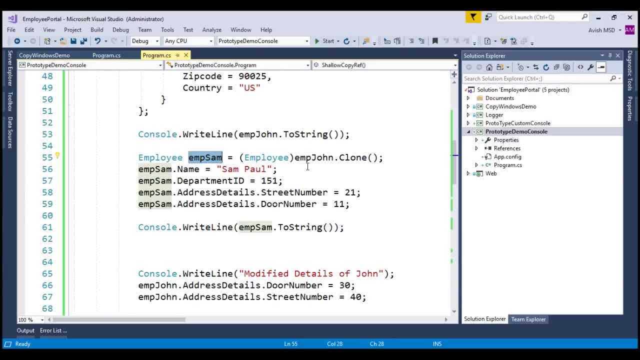 the details to employee sam. object: we are also changing the department id and address details of the sam so that they are different with respect to the employee john. once that is complete, we are printing the details to the console. in step three, we are modifying the address details of the first employee which is employee. 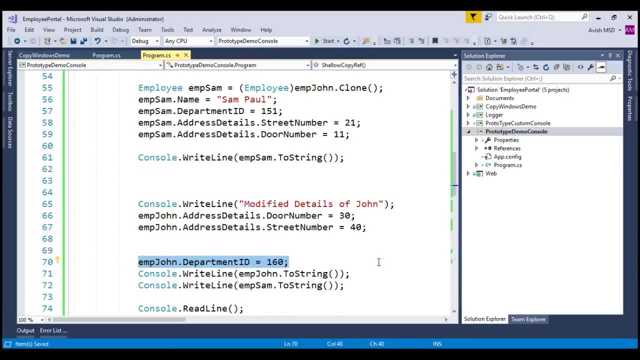 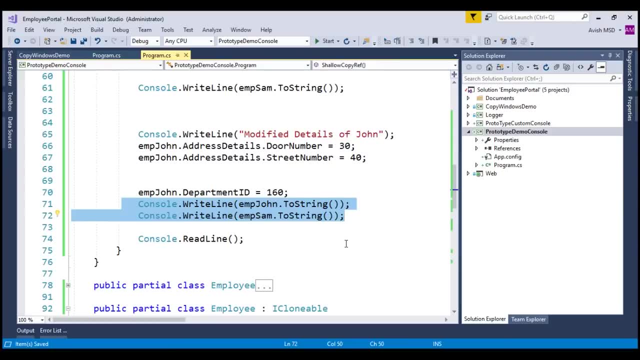 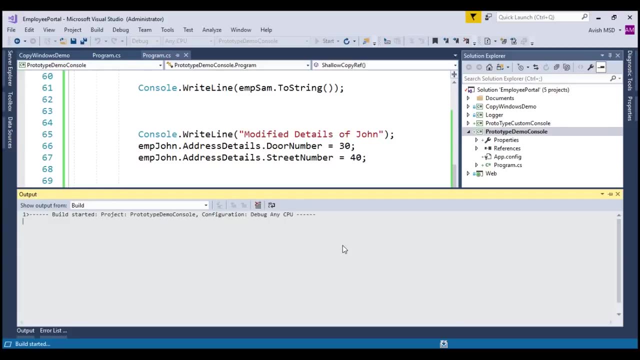 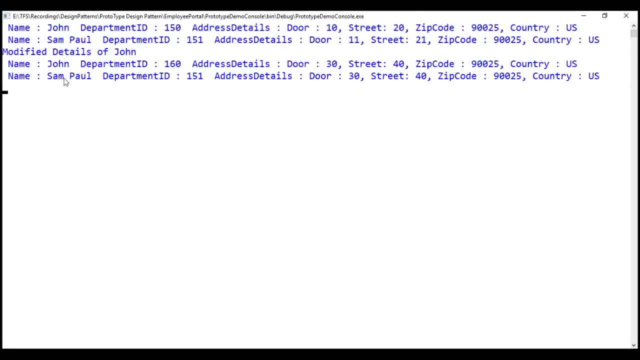 john, we are also changing the department id of this employee. once that is complete, we are printing both employee john and sam's details to the console. let's run this application and see the output. notice that the employee details of sam are changed again, specifically the address details. 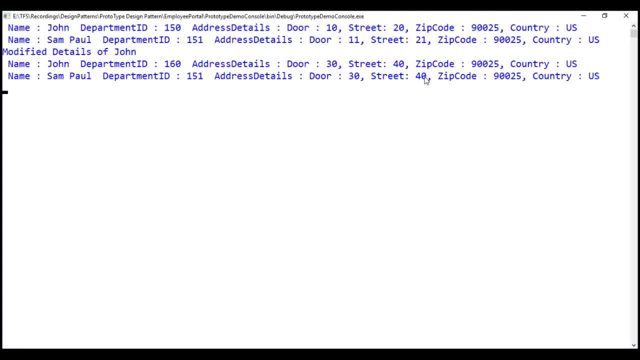 this is because the address is a reference property in the employee object and memberwise clone will copy the reference of the address field, not the address object itself. i hope now you have a good understanding of the memberwise clone and i hope you have a good understanding. 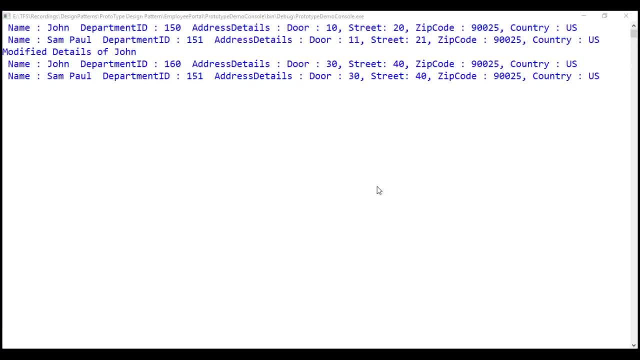 of the memberwise clone and we will see you in the next class. bye, bye. number-wise clone behavior. If you are wondering how to address this situation of reference copying, deep copy would be a solution for this scenario. Again, it depends on your requirement situation if you need to do a deep copy or shallow copy. 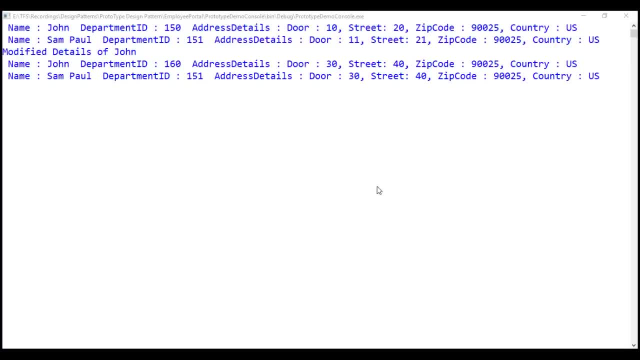 Now assume that the address is the address of the company instead of the employee address. In that situation, shallow copy would serve the purpose, as the company address remains same for all the employees. Let's now switch back to the application and see how we can implement the prototype design. 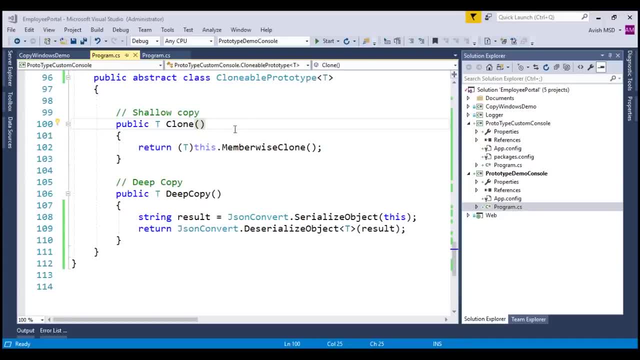 pattern to address both the situations. To make things faster, I have created an abstract prototype class to implement shallow and deep copy. Shallow copy uses the member-wise clone method Which we have implemented in the example earlier, whereas deep copy can be done in many ways.